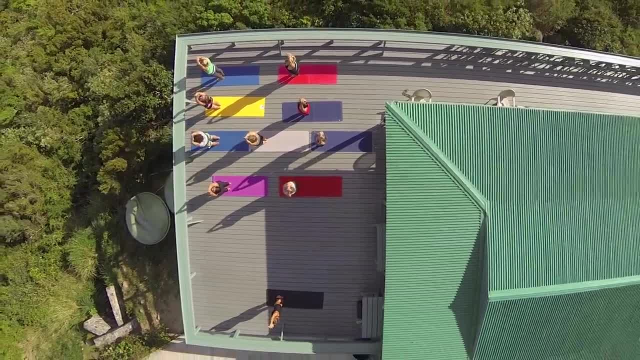 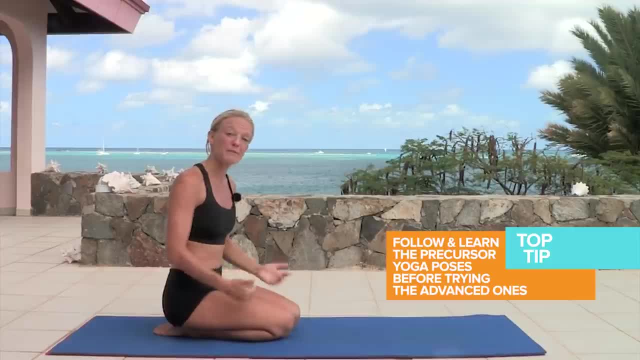 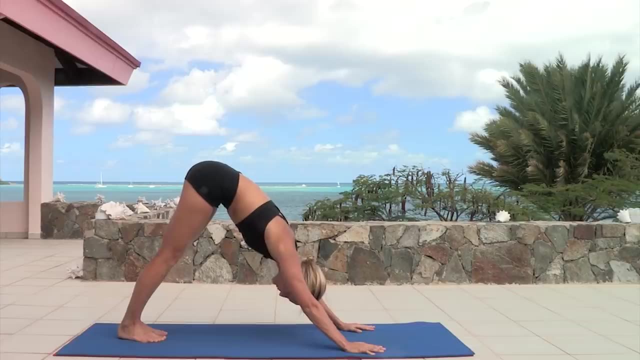 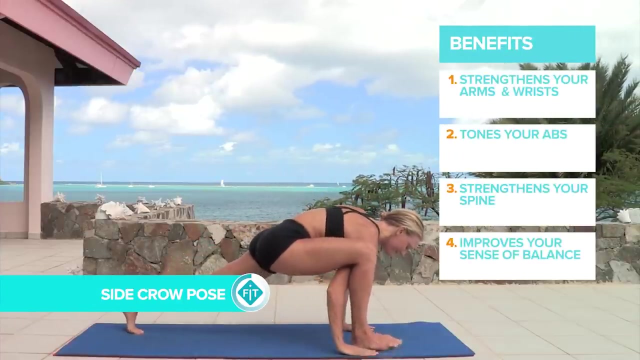 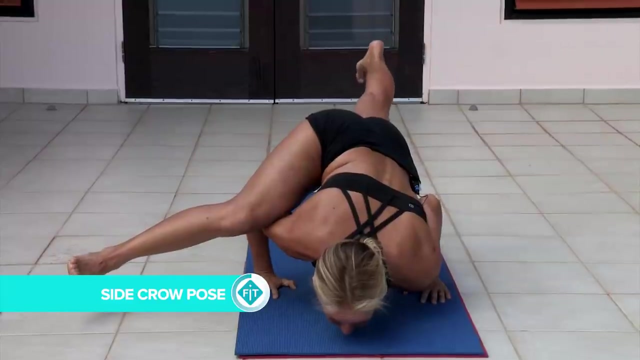 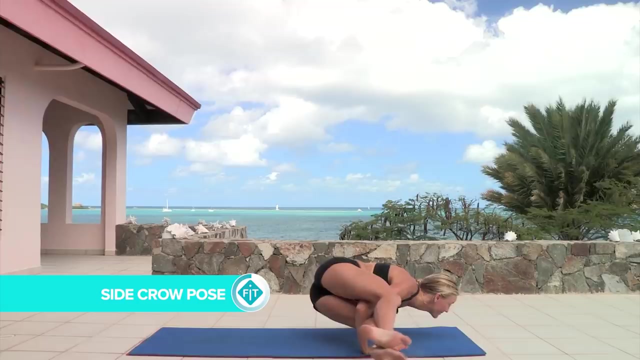 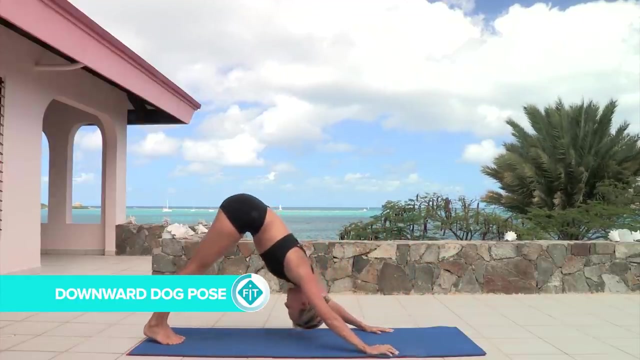 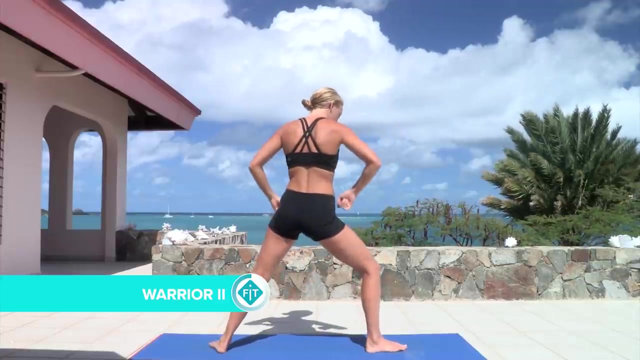 So, with these advanced postures, it's so important to be grounded, to breathe and to, even if the mind wants to do the posture, sometimes the body can't. So to come into Bird of Paradise, I like to begin with a base pose of Warrior II. 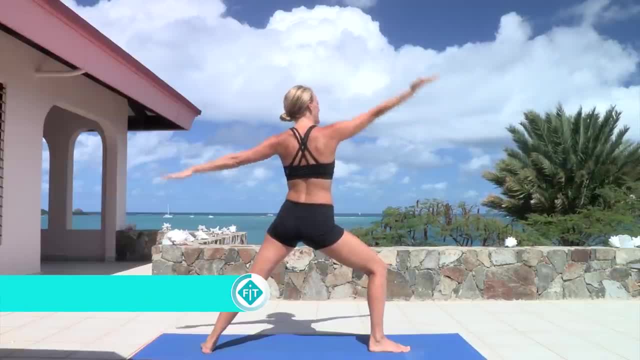 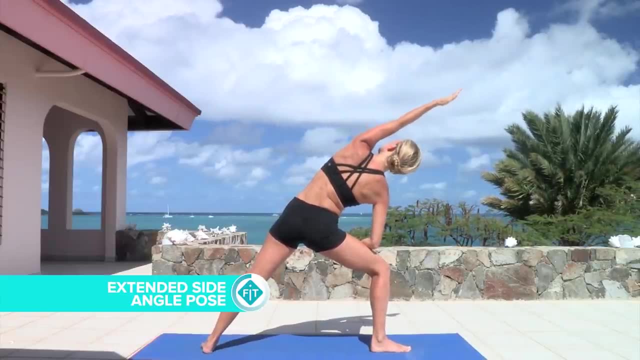 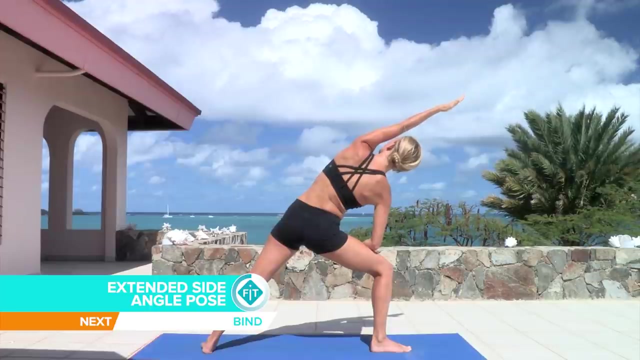 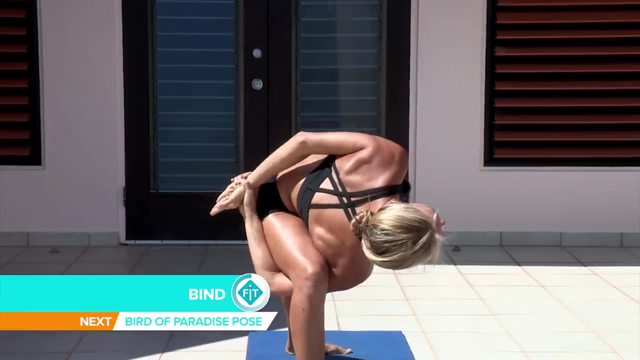 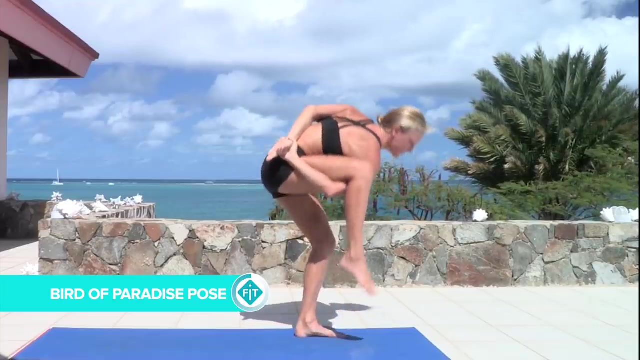 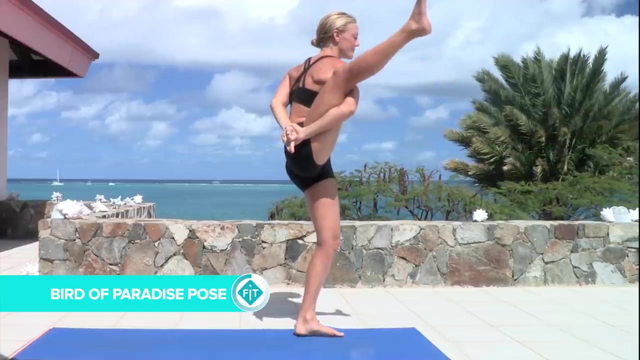 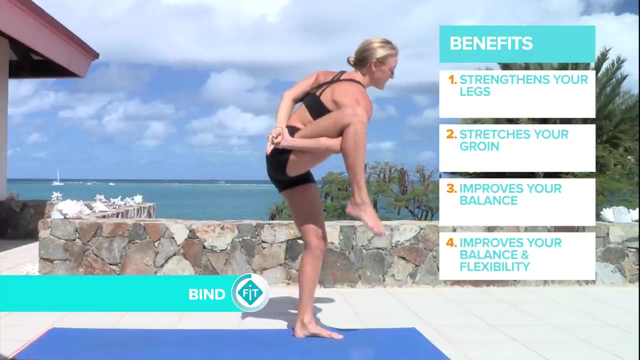 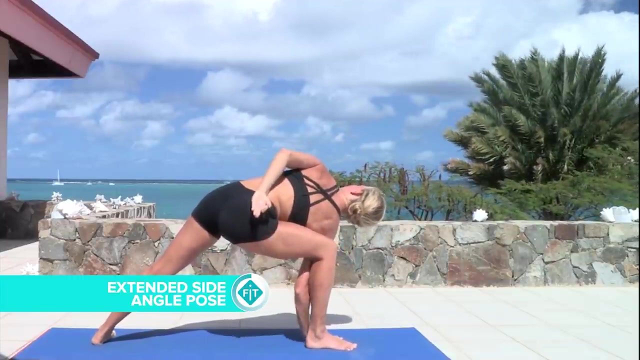 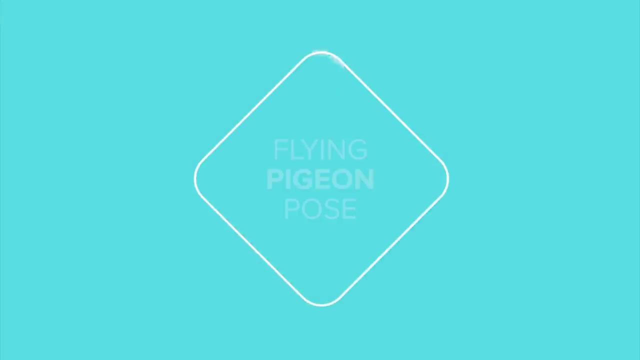 Then we flip the palm into Reverse Warrior, Coming into Parsvakonasana, extended side angle, Breathing deeply. now with Jaya, breath nice and strong, steady, We'll come into a bind. So that's Bird of Paradise. So with Galavasana Flying Pigeon, 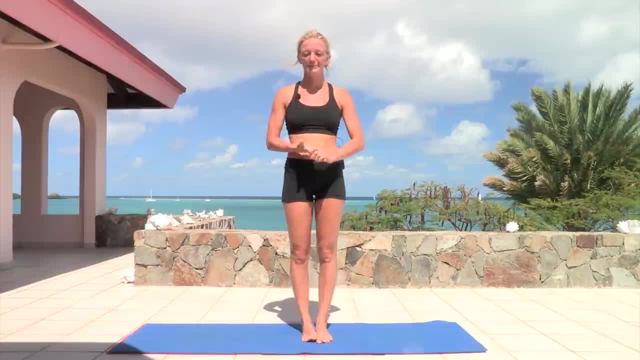 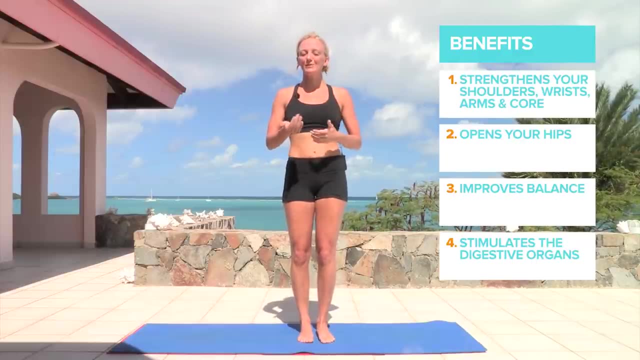 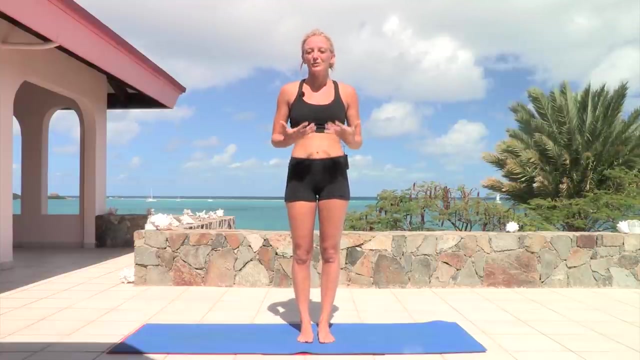 and a lot of arm balances. I find that often you're putting your weight forward, So it's almost you feel like you'd be leaning back because you're scared that maybe you will hit your forehead. But having confidence and faith- these poses are all about strengthening your self-confidence. 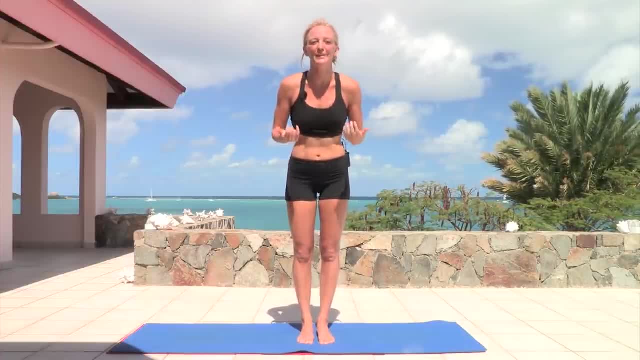 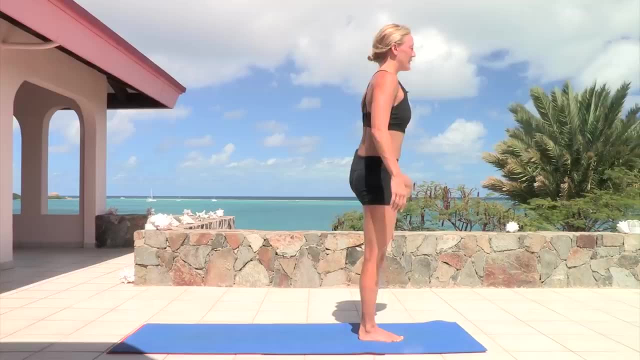 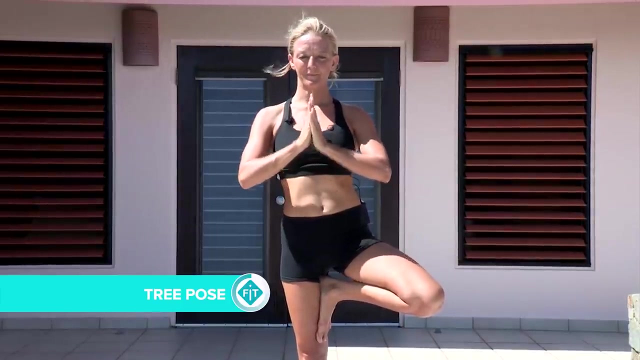 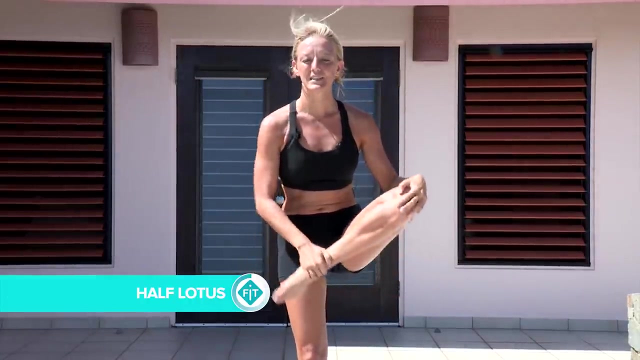 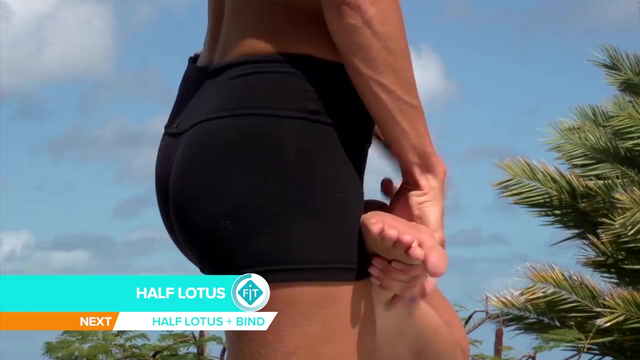 in your own capabilities, so leaning forward. So I like to begin to come into the posture with Tree, Deep breaths And then we go into Half Lotus. So, listening to the knee And bringing the foot nice and close, Come into Bound, Half Lotus. 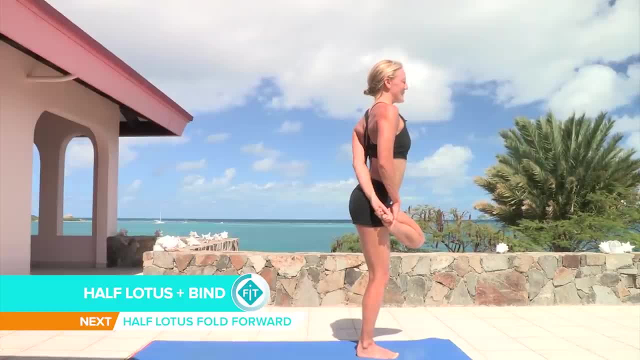 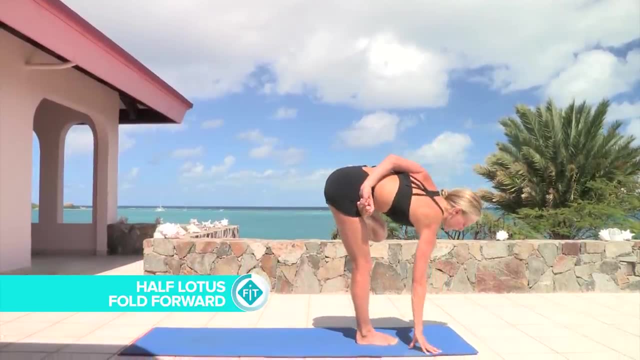 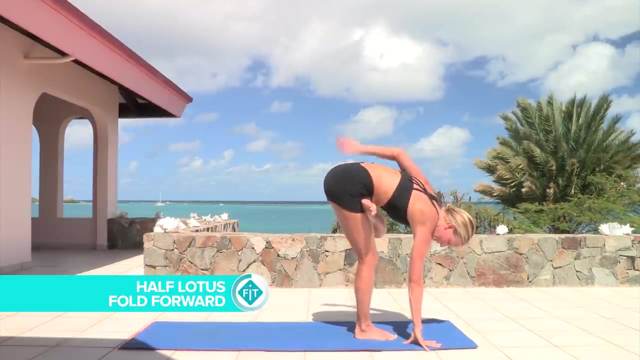 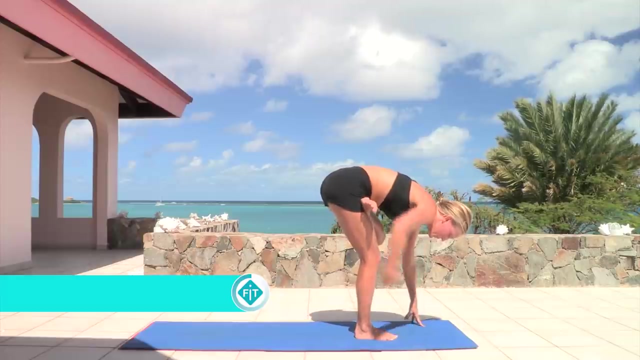 Try to grab those toes, Breathing deeply And then folding forward, And then bringing the other hand down and really folding forward, And then we're going to position the leg so that it can fit into the little tabletop shelf we're going to create with our forearms. 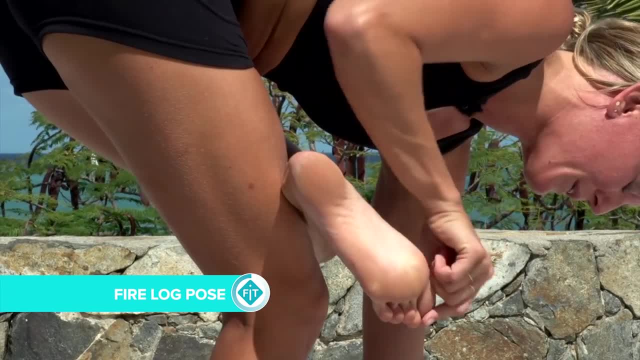 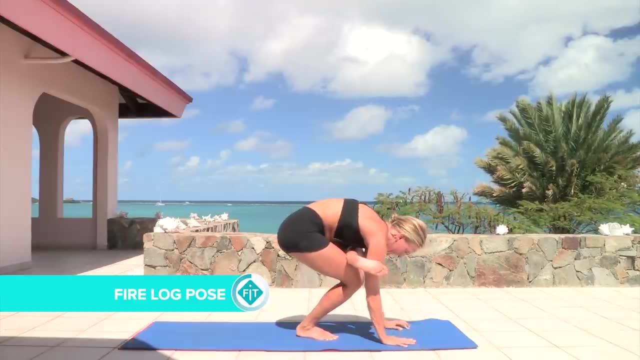 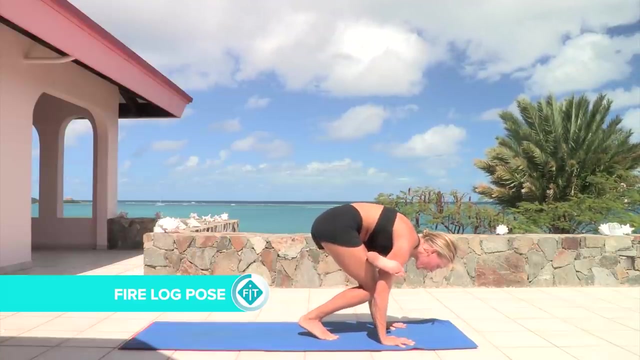 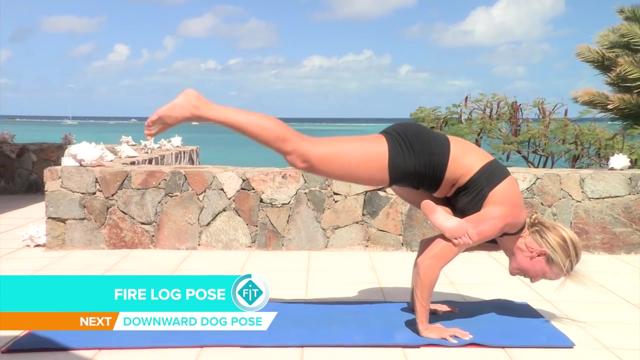 I always flex my foot to protect my knee, So try to bring those toes to touch your shin. Then we step back, Create our little shelf- And here is the key, Where you engage your core And you put your weight forward And you have faith. 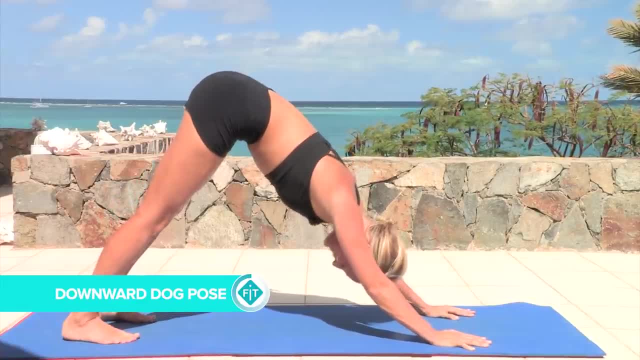 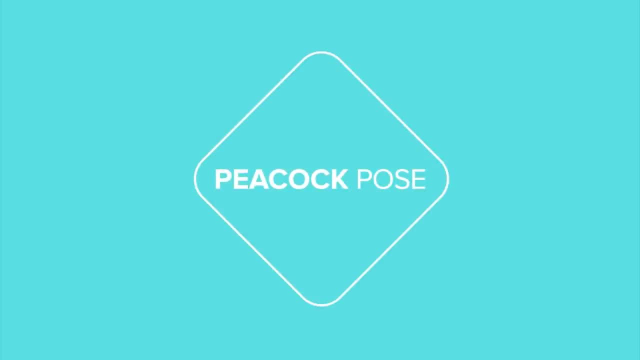 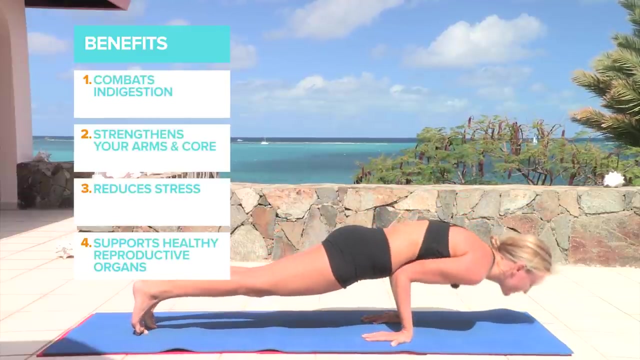 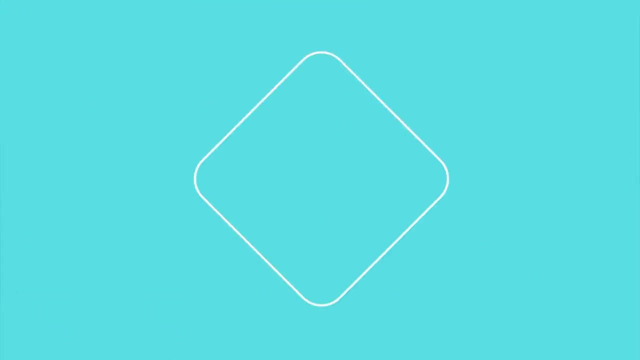 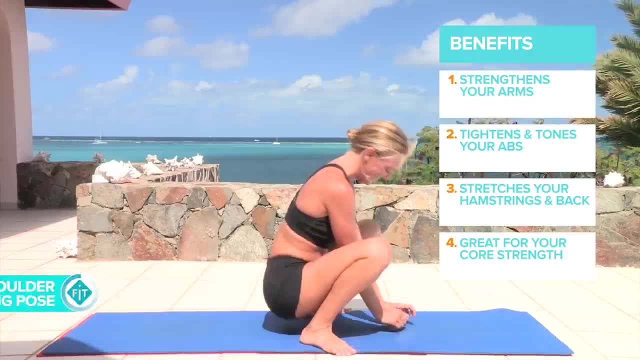 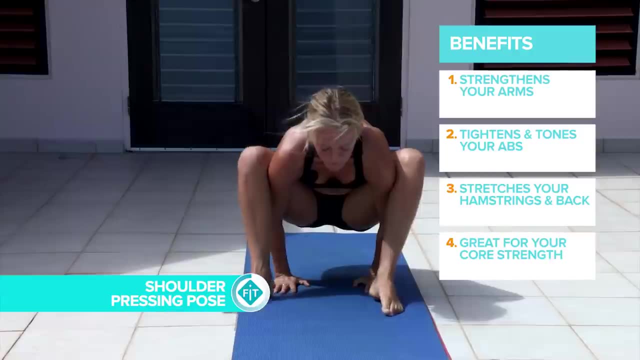 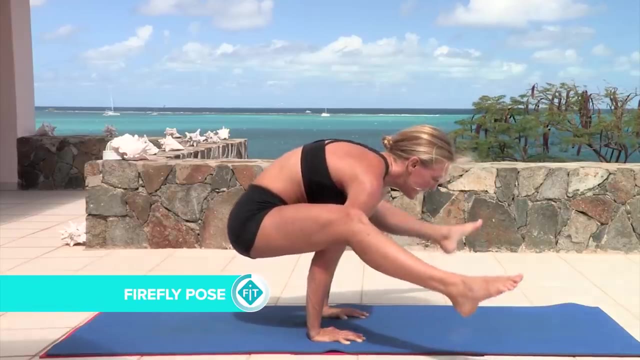 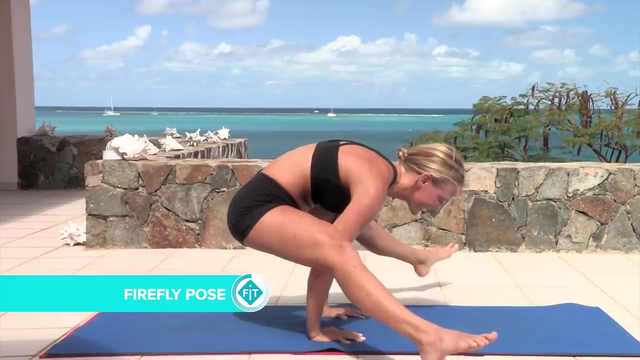 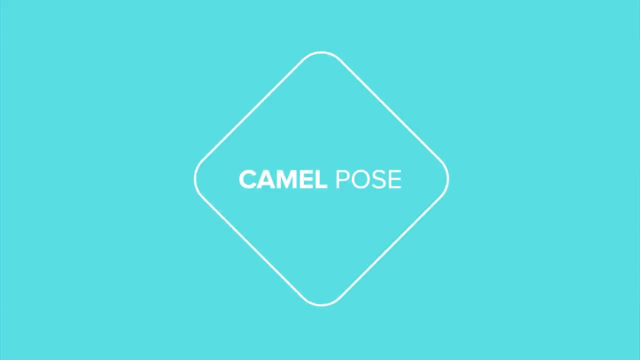 And I will show you Firefly, which is known as Firefly. So first I like to come into this one And from there releasing into this one And leaning forward again, Breathing, Smiling And coming out of it. So the next posture is camel, and I'm going to do a camel drop back. 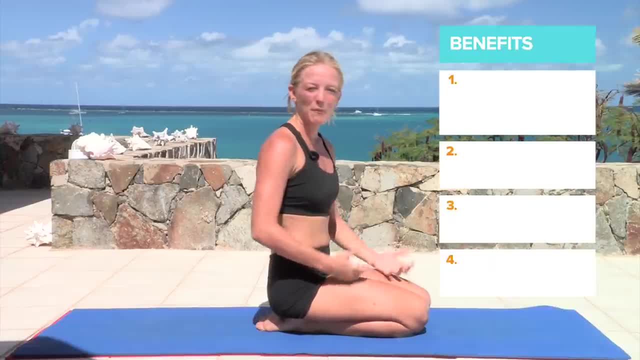 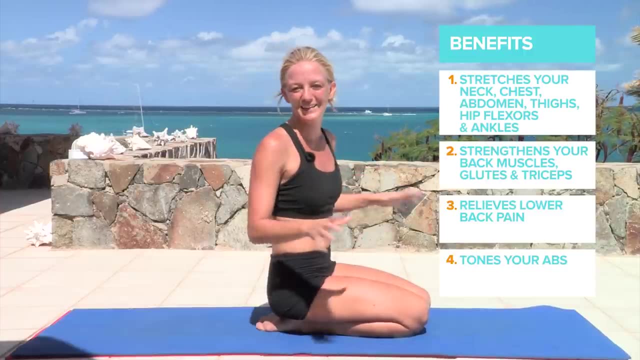 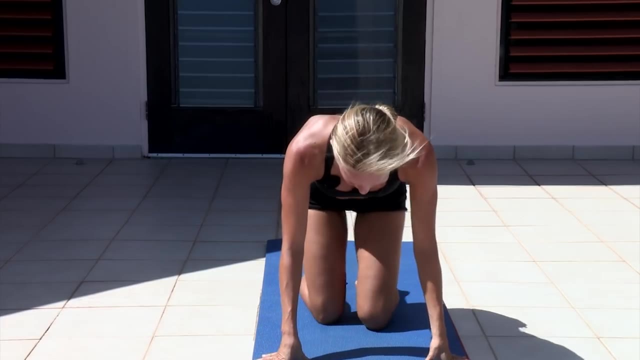 It's called Ustrasana in Sanskrit and with camel you're very opening up your heart. It's almost a vulnerable position because you're so open to the world outside, so I find it important to be in a happy place and a happy state of mind.